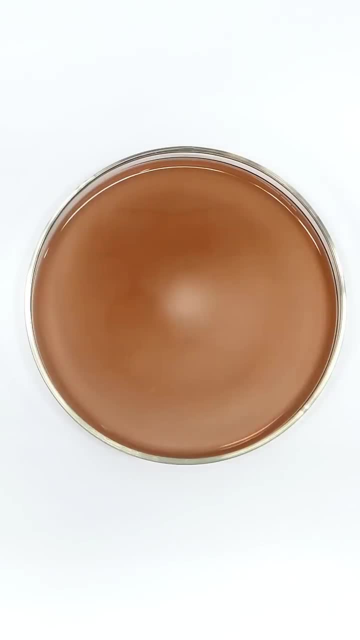 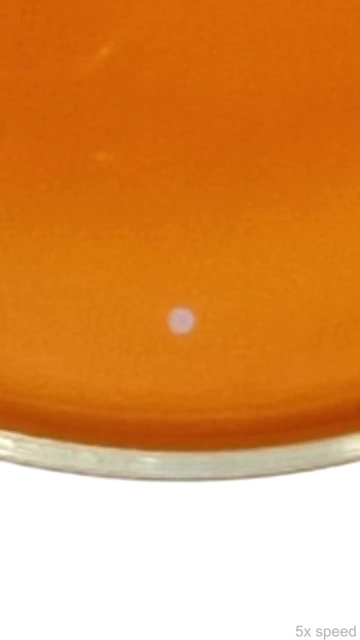 I also have to mix this around until it looks pretty even, and after that I just have to wait. At first, not very much was happening, but then I started seeing some small little spots appearing. Even more of them then started popping up, and they were all getting bigger and bigger. 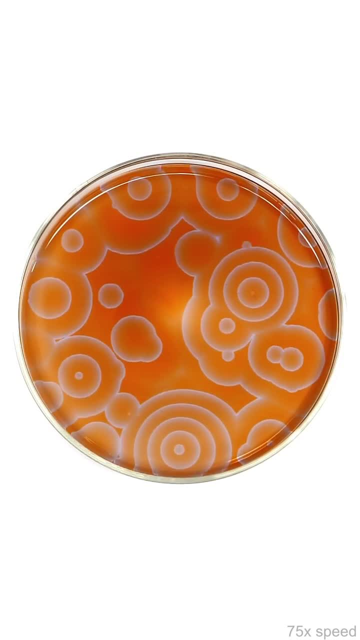 What's going on here is called a Belausov-Zabotinsky reaction, and it's still one of the weirdest- The weirdest reactions I've ever seen. 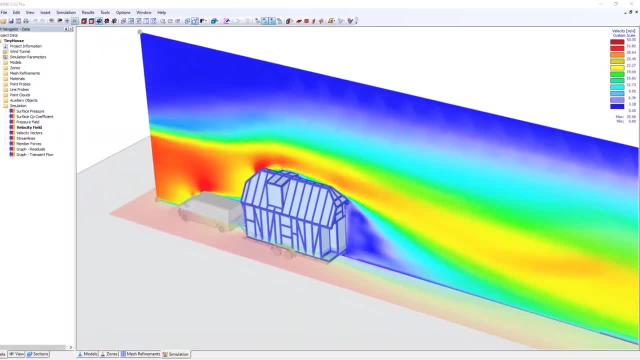 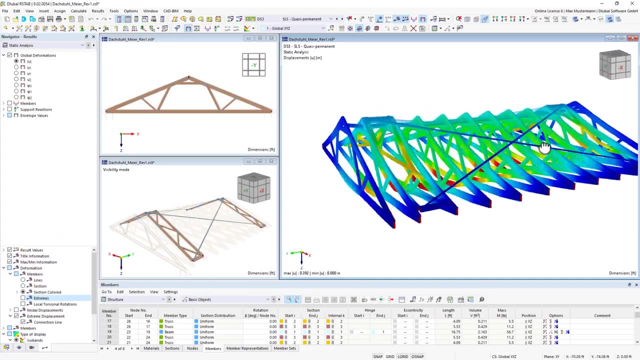 For timber structures. there are many powerful tools in our programs for your daily work as a structural engineer. The best way to design pure beam structures is to use the structural frame and truss analysis software RSTOB9.. If you want to design not only members but also 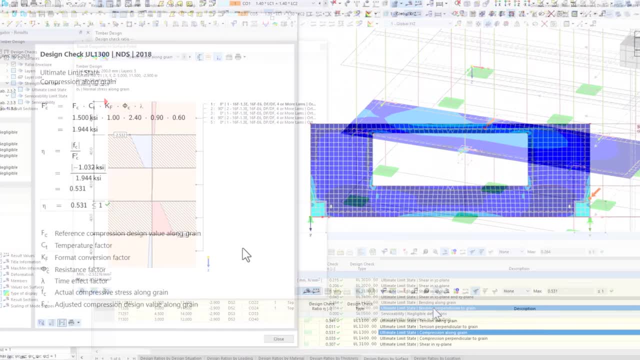 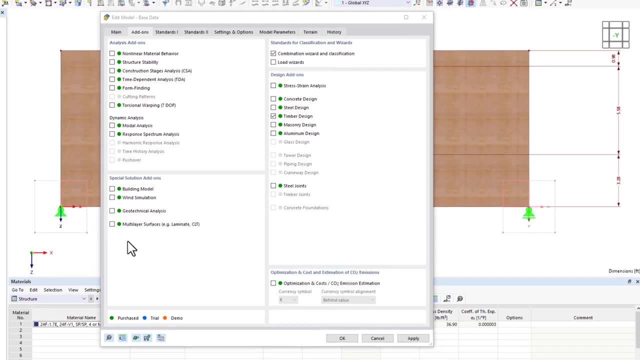 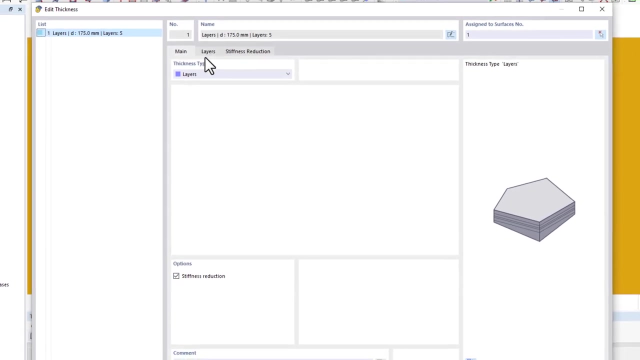 timber surfaces, you need RFEM6.. This means you can also design cross-laminated timber elements In order to use multi-layer surfaces. activate the corresponding add-on, Then you can define the different layers and stiffnesses of the cross-laminated timber elements. 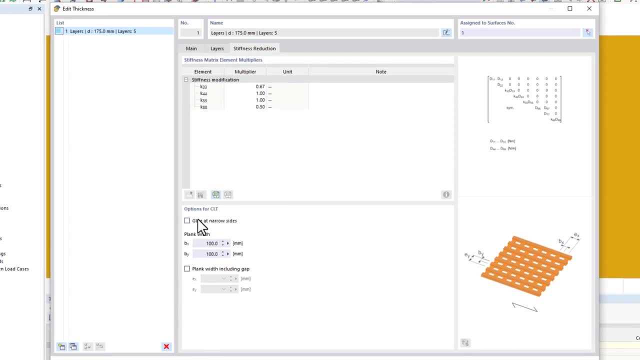 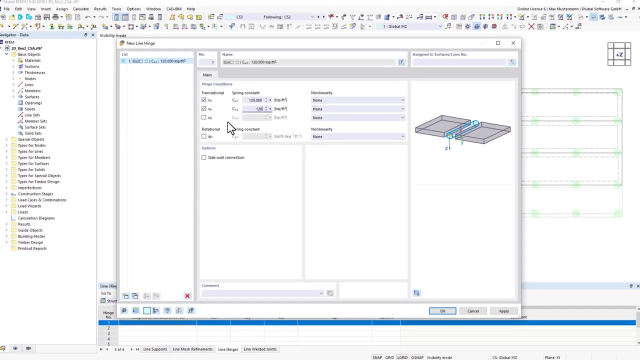 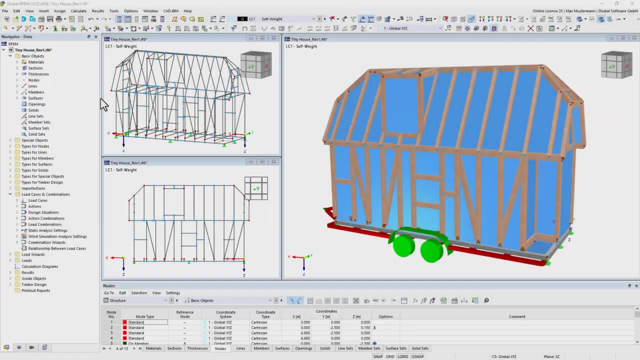 in the thicknesses. End releases of the connections are modeled using line releases or line hinges. Both allow you to exclude or reduce certain degrees of freedom for the transfer. To carry out the design of the structure, you need to activate the timber design add-on and 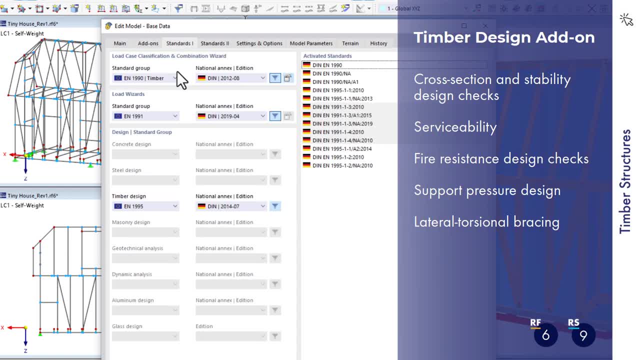 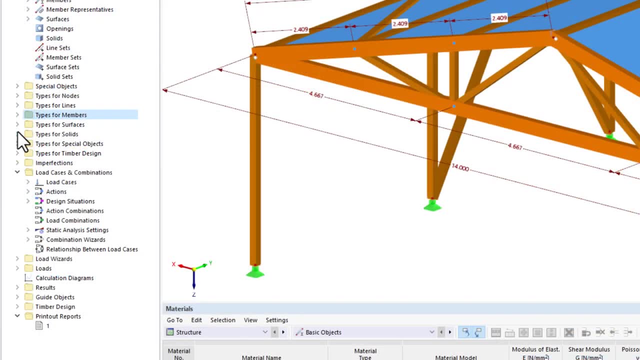 select the correct standards, It is then possible to carry out the design of the structure, to carry out the ultimate and the serviceability limit state design, as well as the fire resistance design of all timber components. After activating the add-on, dialogue boxes appear where you can.